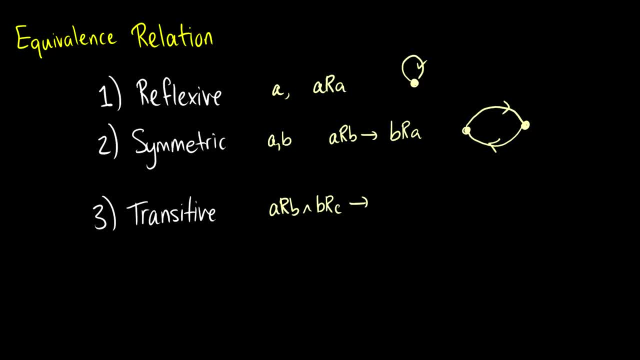 if b is related to c, then we're going to get that a is related to c. So we have three points here and we have an arrow from a to b. we have an arrow from b to c. therefore, we're going to get this arrow from a to c. So when we put the three together, let's say: 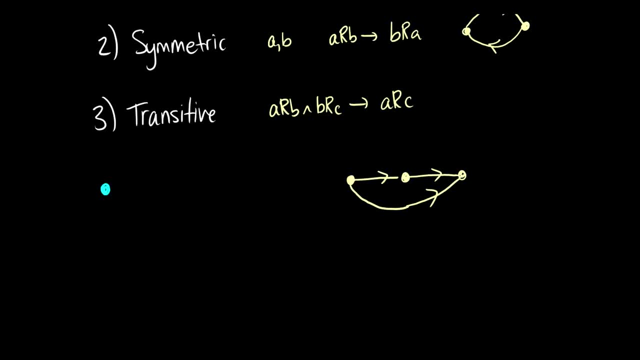 we have three elements, So we have these three here. Well, they all have to be related to themselves. So we get some nice reflexive arrows here, And let's say that a is going to be related to b, So we'll have this arrow going here. 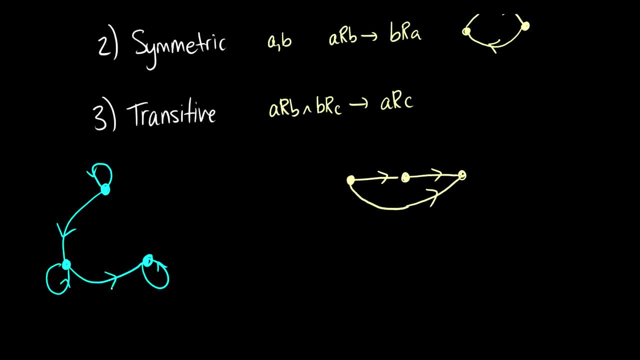 We're going to have b related to c, And now, if we have this graph, that means that, well, if we have an arrow pointing from one node to another, by symmetry we have to get arrows pointing back, And by transitivity we have to get arrows pointing back. So we have a. 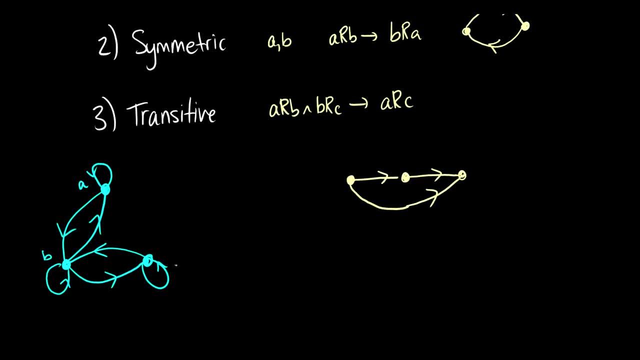 because this node a points to b and b points to c. then we should get an arrow from a to c And by symmetry we get an arrow back, So we get this super looped crazy thing, And basically what this says is that all of the elements are equal to each other. So a good 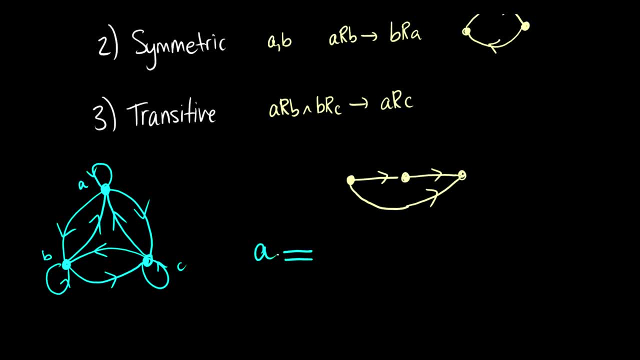 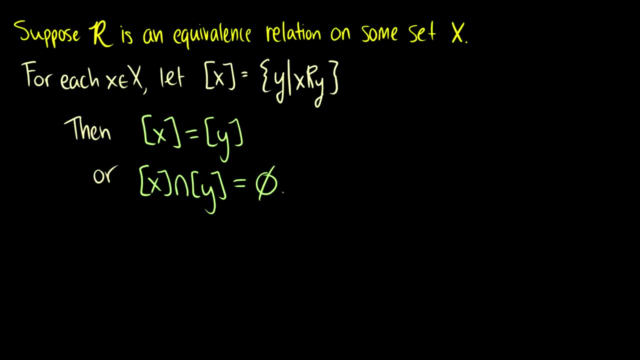 equivalence relation is the equal sign. So a is equal to b is equal to c, And we get: a is equal to c, So 1 is equal to 1 is equal to 1.. This satisfies all three conditions, But we've already talked about that, So let's go on to denoting equivalence relations with: 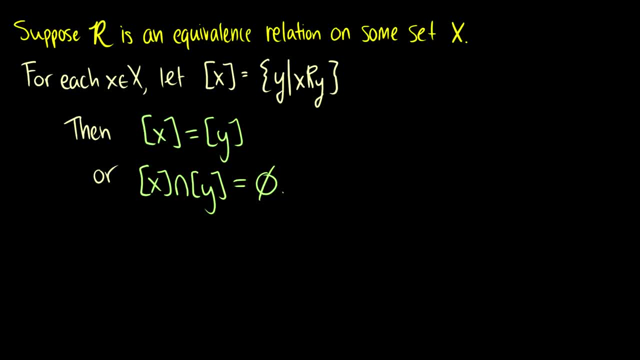 notation. So we can write an equivalence relation r as this sort of box x. So we say x in square brackets And it's equal to the set of y, such that x is related to y, So it's equal to the set of y. So what this means here is if we have some element a and we have another element, 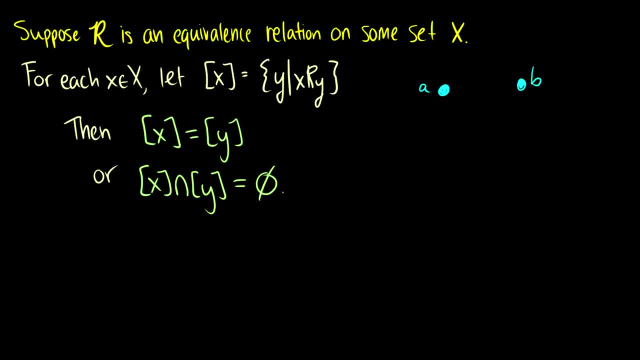 b. then the equivalence relation on this element a. here is everything that's related to b. So let's call this box a, for instance, And we say that a is related to b, This means that this is just the set b. So this might be a little bit confusing, but these two points. 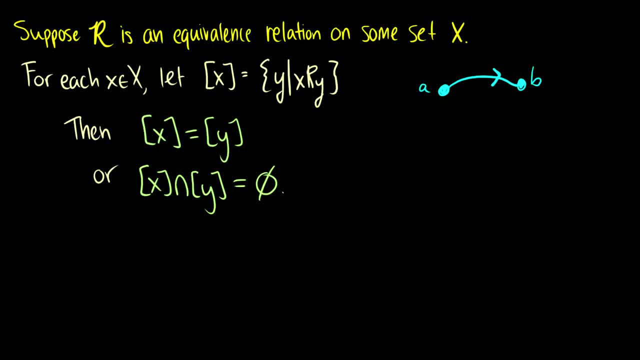 coming up next are going to hopefully clear it up a little bit. First point is: either the equivalence relation on x can be equal to another equivalence relation, y, or the intersection of them can be empty. So basically what this means is, let's say, if we have a is related. 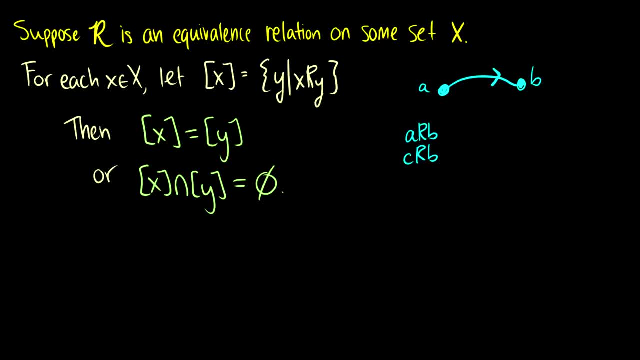 to b and c is related to b. Well then, we have this condition here where the equivalence relation of a is going to be the same thing as the equivalence relation of c, But let's say a is related to b and c is going to be related to d, And we know that a is. 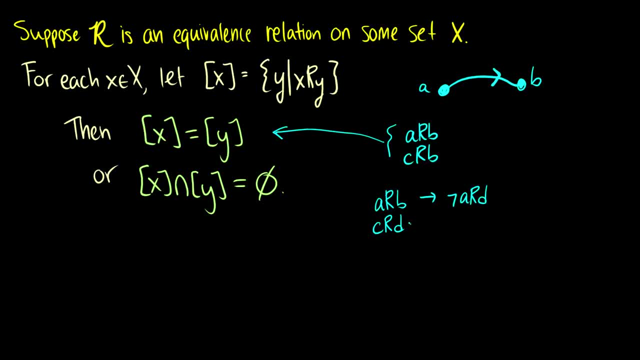 not related to d. This means that c cannot be related to b if we have an equivalence relation, because their intersection must be empty. So you don't normally see this notation used too much. But if we have an equivalence relation, then we know that a is not related. 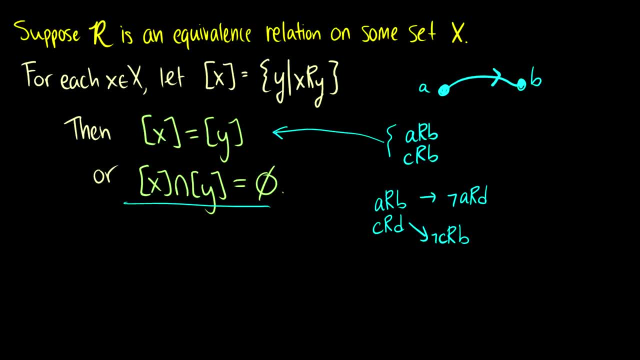 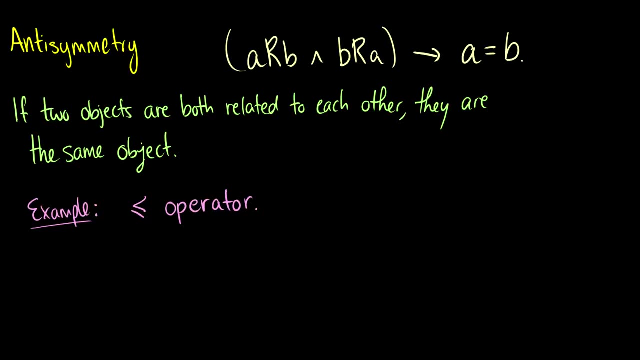 to b. So this is a good idea to introduce it now, just to get it into your minds. So we need to introduce a new type of relation and that is the relation of anti-symmetry. Now, when you see the word anti, you sort of think of the word not, And we should not do. 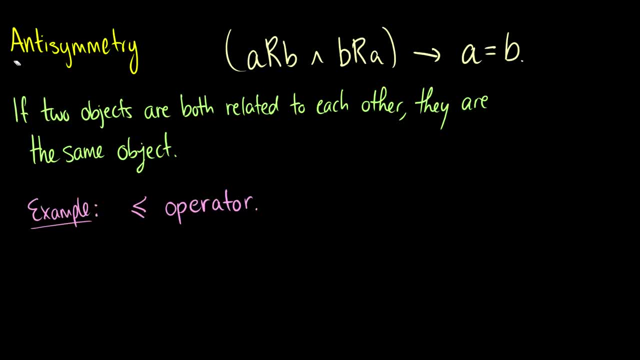 that with anti-symmetry, because the definition is a little bit more confusing. So what this says is that if a is related to b and b is related to a, then a is going to be equal to b. So what this means is that if two objects are related to each other, 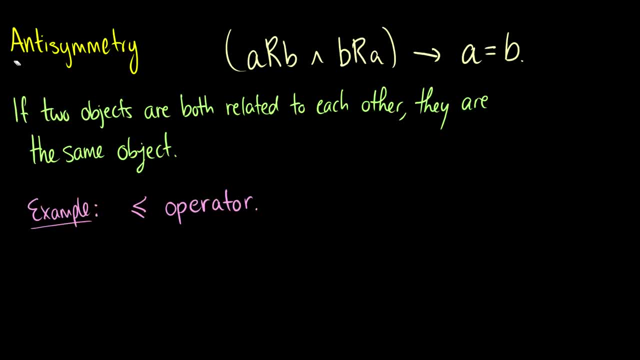 they're going to be the same object in an anti-symmetric relation. So for instance, we have this: less than or equals to sine operator. So if we have the case where x is less than or equal to y and we have the case where y is less than or equal, 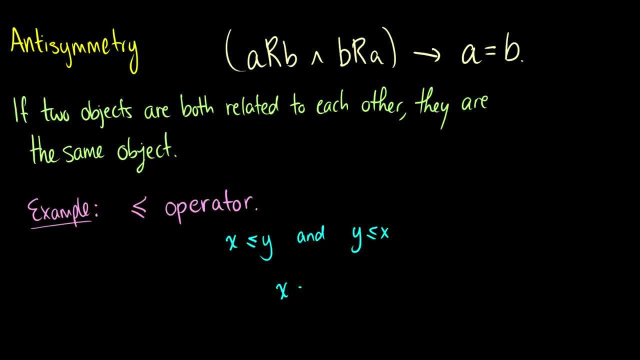 to x, Then we're going to get that x is equal to y, Because that's the only way that these two values are going to make any sense. x has to be equal to y, And another operator we can show this with is the subset relation. 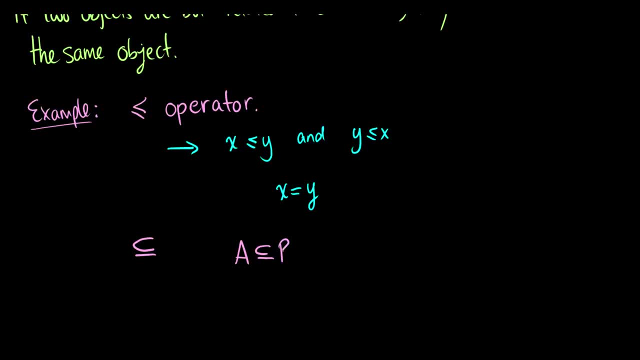 So if we have a as a subset of b and we have b is a subset of a, then we know that the the sets A and B are equal to each other by definition, because all of A is contained within B and all of B is contained within A. Therefore they must both be equal. So this is the anti-symmetric. 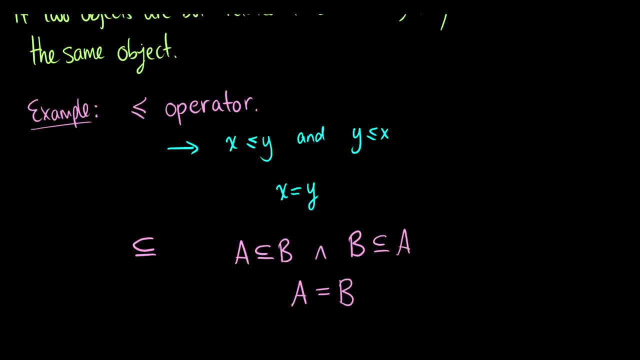 property, And we're going to be using this in the case of partial orders. So partial orders, they are not an equivalence relation, but they're another type of relation that we should be familiar with. So a partial order is going to be anti-symmetric, So no surprises there. 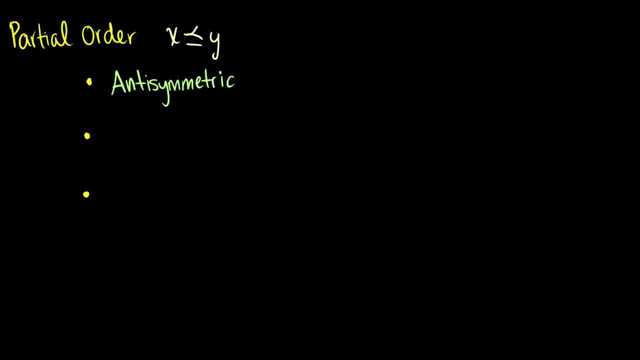 If there was a surprise, well, I wouldn't have introduced anti-symmetry in the slide before this. It's going to be reflexive and it's also going to be transitive And with partial orders. what we can do is we can use this little symbol right here, sort of like a 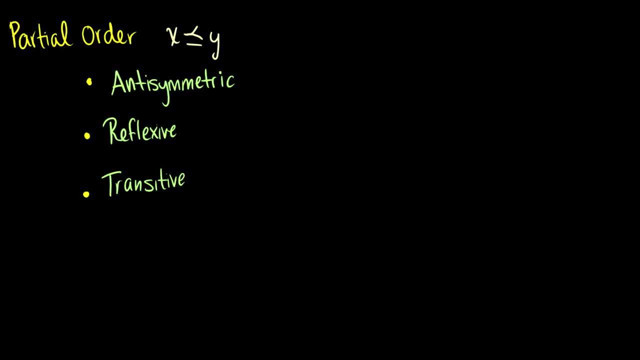 like an like, an like an less than or equals to sign like a little tail sticking out. Not really, but we can use that to denote a partial order And basically what we get with a partial order is we don't get the case. 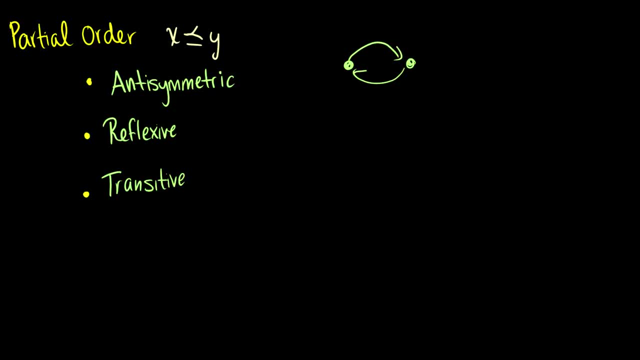 where, if we have two elements, they go back and forth. We don't get this property. Instead, what we get is this sort of property- And I'm going to hold off on that sort of explanation for just a second here- And we're going to talk about some types of partial orders, because I think it's good to do this before we get into how we show them graphically and how we talk about them. So here's a couple types of partial orders. We have x less than or equal to y. So this is sort of true. Well, it is true, completely true. Suppose we have, say, two elements. 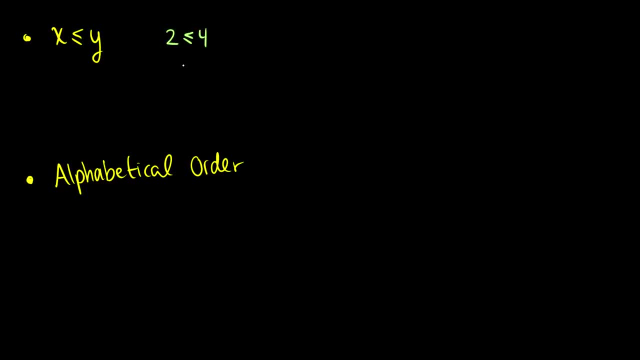 Well, it's reflexive. And so, for instance, we have two less than or equal to two. This is going to be true for any element. It's transitive, because if we say, have a two less than or equal to four and we have four less than or equal to five, then we know that two is going to be less than or equal to five. And it's anti-symmetric, because if we have 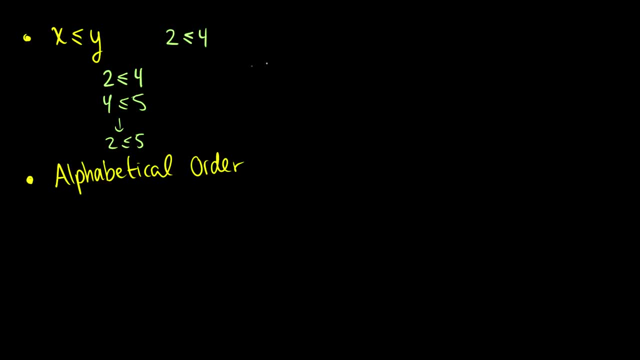 three is less than or equal to three, or let's just say more generally, x less than or equal to y and y is less than or equal to x, then we're going to get x is equal to y. So that's a partial order. Alphabetical order: it's a little bit more interesting, but it's basically the same system as the x less than or equal to y order. Instead of looking at values of numbers, we just take the letters in alphabetical order. So we know that a is going to be 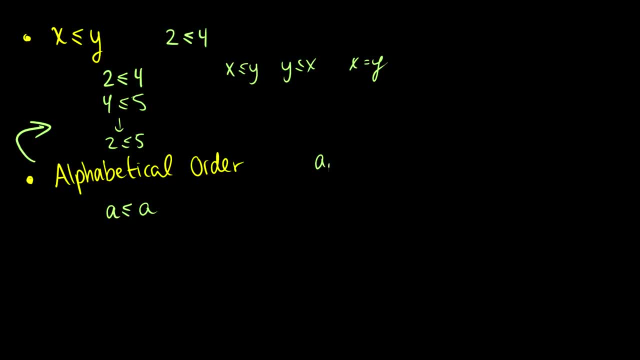 less than or equal to a. If we order it like a, b, c and we call that an ordered pair and that's the whole alphabet goes down to z, then we know that a is going to be less than or equal to the position of a. If a is before b and b is before c, then we know a is before c. And if some letter x is before the letter y or at its position and y is, 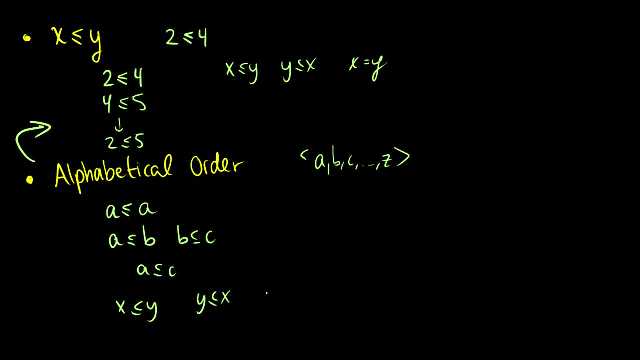 before at position x, then that means that x must be the same thing as y, So it's a little bit more abstract there, but we can write this using our notation as a is in a poset or a posit with respect to b, c, so on and so forth, So we can show partial orders like this. Now, a good way to represent. 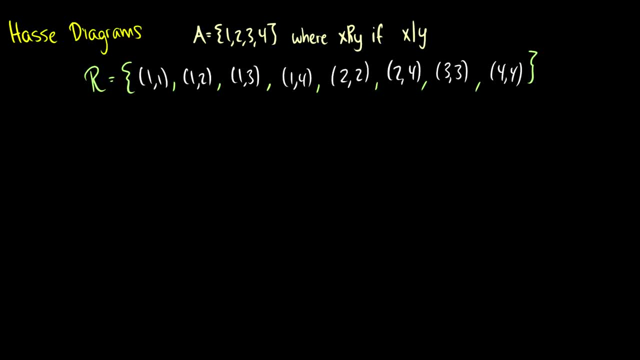 partial orders is with Haas diagrams or Haas-y diagrams. So we have a set here- 1, 2, 3, 4, and we've defined a relation where x is related to y if x divides y. So x exactly divides y. So if we take a look at our relation here, 1 divides 1, so you can put 1 into 1.. 1 divides 2,- you can put 1 into 2.. 2 divides 2, because you can put 2 into 2.. 2 divides 4, because you can put 2 into 4 twice. 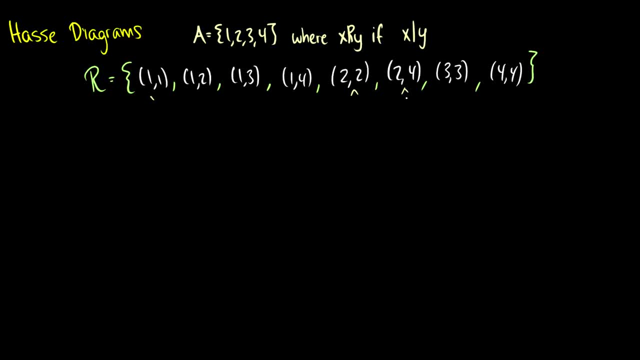 2 as 7. And 2 as 7. And so on and so forth. So this is the relation we're going to look at, And we should probably check to see if it is in partial order. So let's take a look here. Is it reflexive? Well, we have 1, 1, 2, 2, 3, 3, and 4, 4, so we're good. Is it transitive? 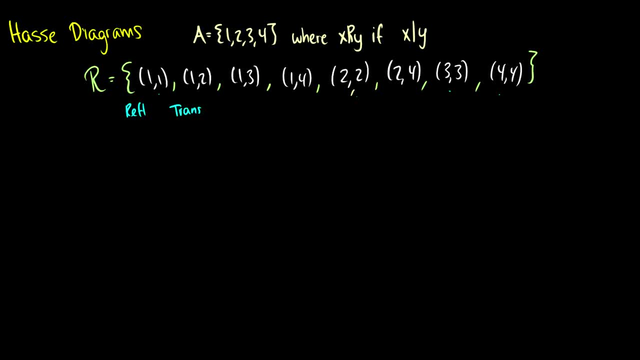 Okay, well, we have 1, 2, and 2,, 2, 4, so we should have 1, 4.. Okay, we're good And we have. I think that's really it we have to look for in transitivity. 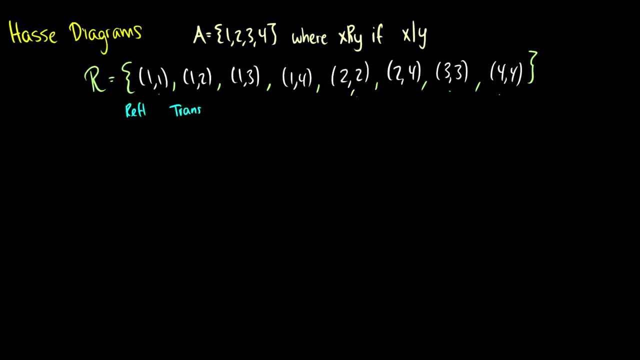 And then anti-symmetry. Basically, do we have two things that are symmetric to each other? We have 1, 2.. We don't have 2, 1.. We have 1, 3.. We don't have 3, 1.. 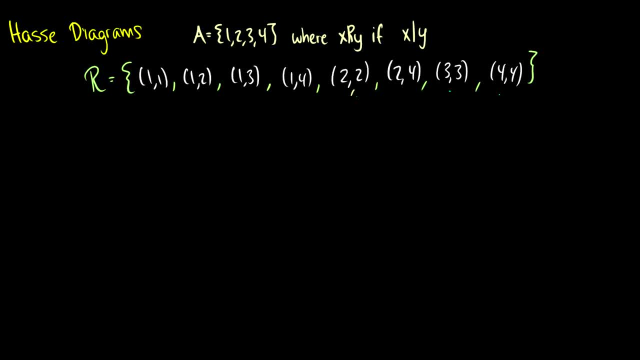 We have 1, 4.. We don't have 4, 1.. 2, 4.. We don't have 4, 2.. So, yeah, we're looking good here And, of course, symmetry is okay because we have 1, 1.. 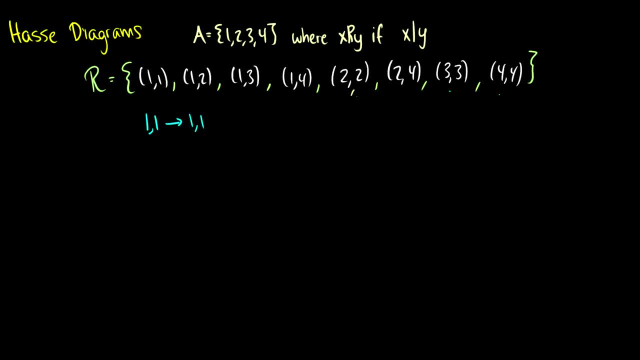 So it's also going to be 1, 1.. Because if we have 1, 1 and 1, 1,, then 1 is equal to 1,, which we know. So how do we represent this? Well, what we do is we give each element a point. 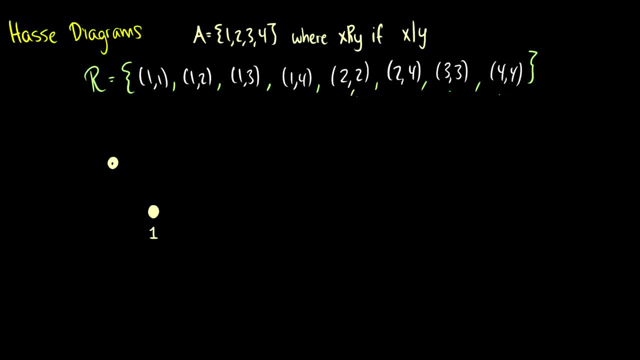 So we'll call this 1.. I'm going to put 2 over here, Put 3 right here And let's put 4 right up here. So we're going to draw some arrows with our relations here. So we know 1 goes to 1.. 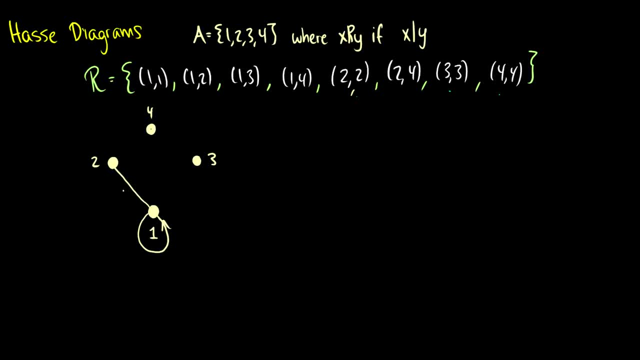 So we'll put an arrow there. 1 goes to 2.. 1 goes to 3.. 1 goes to 4.. 2 goes to 2.. 3 goes to 3.. 4 goes to 4.. And we also know that 2 goes to 4.. 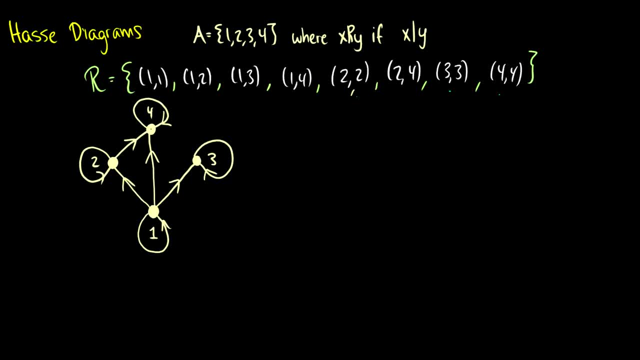 So we have this diagram here and it's pretty messy. So we have these wonderful things called Haas diagrams that make things look just a little bit nicer. So here's what we do: When we do a Haas diagram, we say it's a partial order. 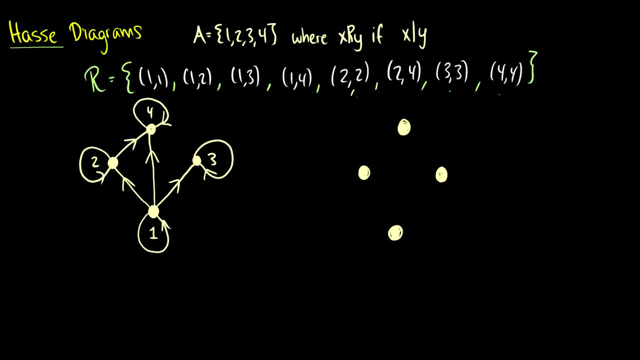 since we only use Haas diagrams for partial orders. So there's a few things we know. Let's just label these: 1,, 2,, 3, and 4.. We know in a partial order everything is going to be symmetric. 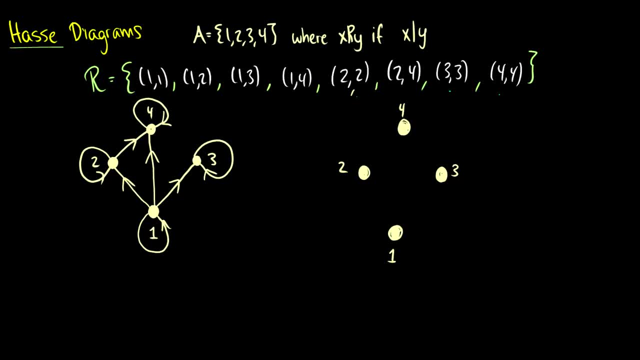 So what we're going to do is just eliminate all of these. We're going to eliminate all of our reflexive arrows. We also know that in the case where 1 goes to 2 and 2 goes to 4, we're going to get this: 1 goes to 4 by transitivity. 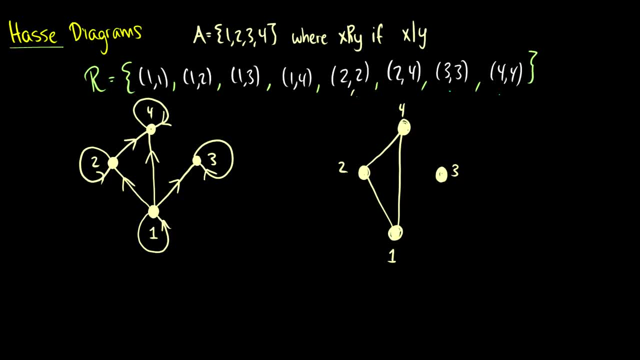 So instead we're just going to say: well, we know it's going to be transitive, so let's just eliminate that line. We don't need that either. In fact, we're going to eliminate direction completely, because we can figure out the direction it goes. 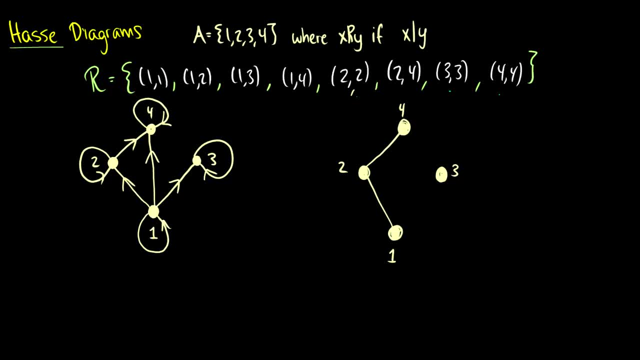 and we know it's always going to be in the same direction due to the anti-symmetry property. So when we do all of that, we remove the reflexivity, we remove the transitivity, we remove the anti-symmetry from our diagram. we get something a little bit cleaner. 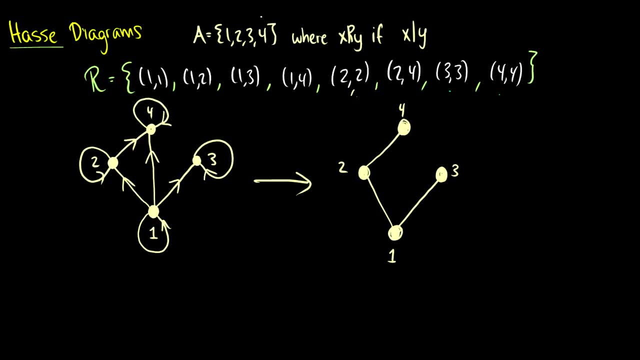 And basically what this means is that we have well the same relations that occur over here, just we've made it a little bit nicer. So if we have a path from 1,, 2, and 4,, this means that we have 1, R 2, 1, R 4.. 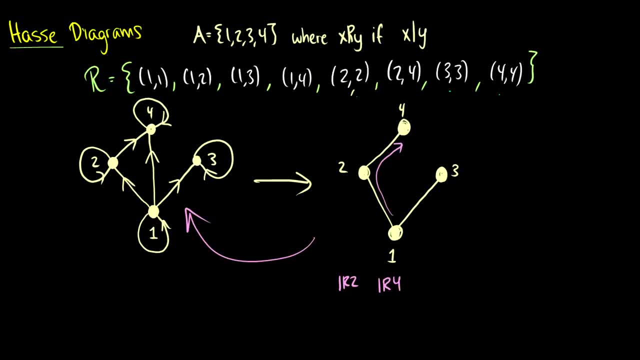 So if we connect something to a higher element, it's in a relation with everything it's connected to. So 1 is in a relation with 3,, 2 is in a relation with 4, and it's always going to go up. 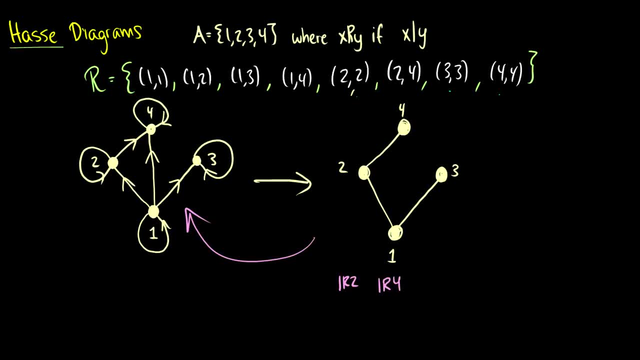 You can draw them from top to bottom or bottom to top. It's good to specify which general convention is that the lowest number? and it's always going to go up. So if we draw them from top to bottom or bottom to top, it's good to specify which general convention is that the lowest number? 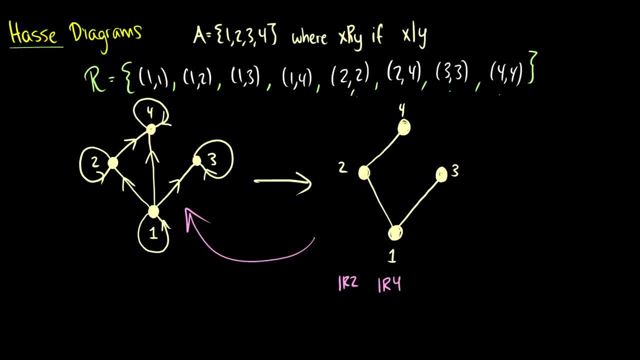 goes on the bottom and it works bottom to top. So that's a Haas diagram. It's kind of nice to look at. It's a little bit cleaner. Eliminating arrows is always a nice thing to do, So there's a very interesting type of Haas diagram. 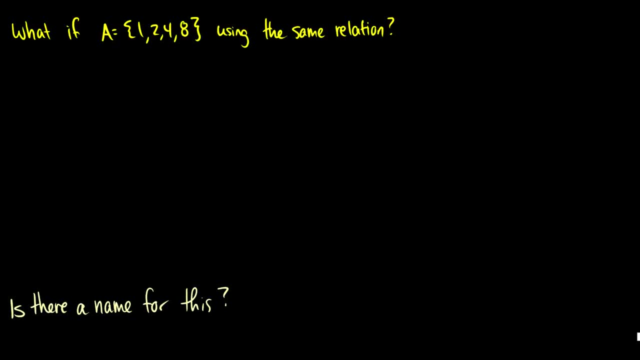 and I'm going to demonstrate it with this set: If A is 1,, 2,, 4, and 8, and we're going to use the same relation that X R Y is if X divides Y. So what's interesting about this? 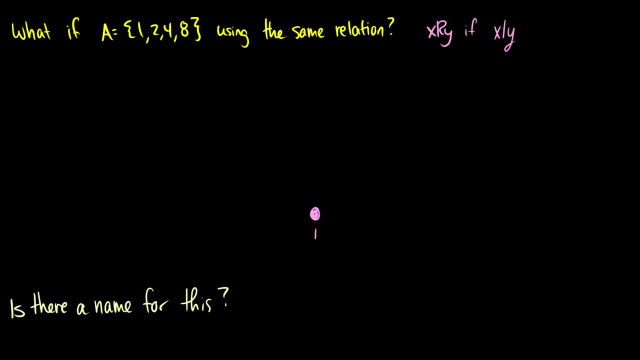 Well, 1 divides 2, 1 divides 4, 1 divides 8.. 2 divides 4, 2 divides 8, 4 divides 8. And of course they're all reflexive. we know that. 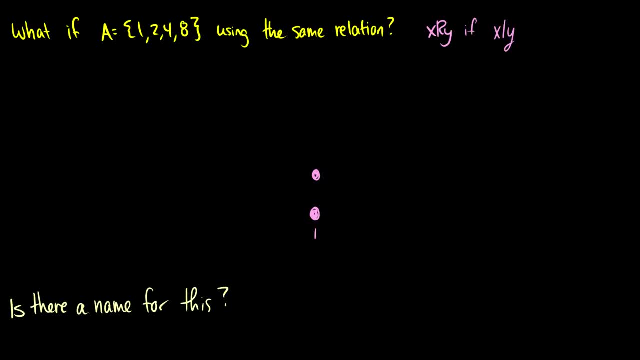 So let's draw what this will look like. So I need to be pretty careful here, Because we're going to do it without a Haas diagram and then we're going to do it with a Haas diagram, So we'll do that. 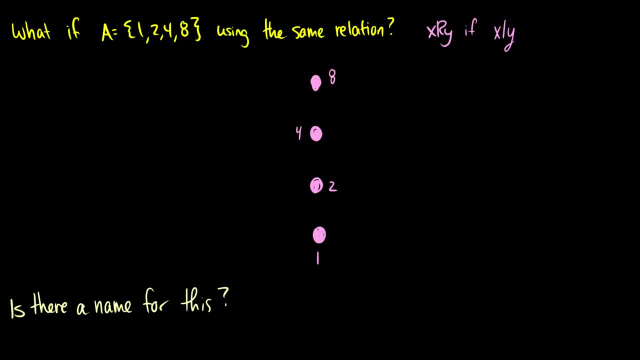 That should be a 4, and that should be an 8.. So we know all of these are going to be reflexive, so we're going to have to draw some reflexivity in there, And 1 is going to go to 2,, 2 is going to go to 4,. 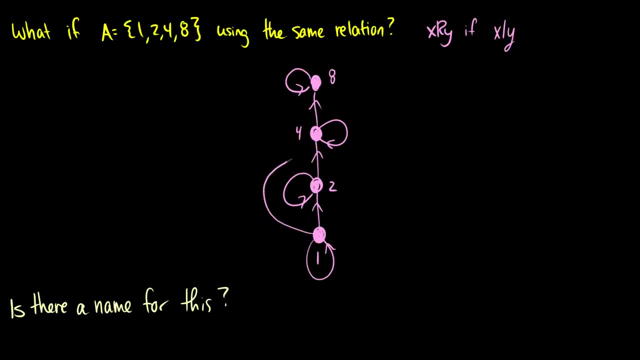 4 is going to go to 8.. And we also know that 1 is going to divide 4, and 1 is going to divide 8.. We know 2 is also going to divide 8, and it's going to be a little bit difficult to make this look good. 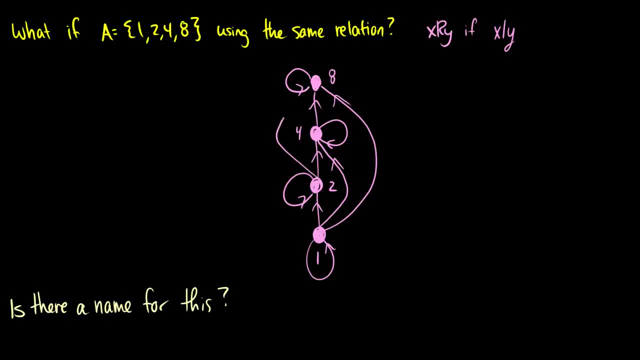 So I'm going to put this in there. and 2 divides 8. And this looks like just a terrible mess. So let's reduce this to a Haas diagram. Well, we'll get rid of reflexivity here, because it takes up a lot of space. it's kind of ugly. 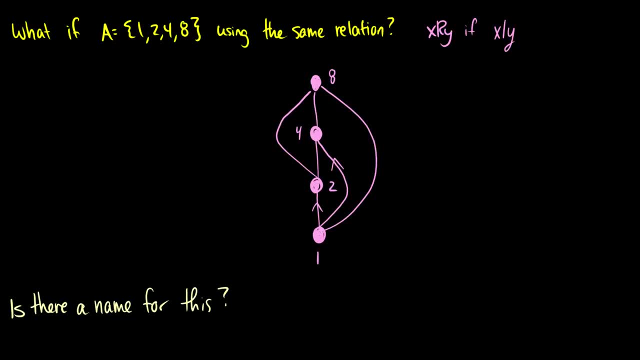 We're going to get rid of our directions on all of our arrows because they're not necessary, And we're going to get rid of transitivity because we know that all partial orders are transitive. So now we get this really nice diagram. 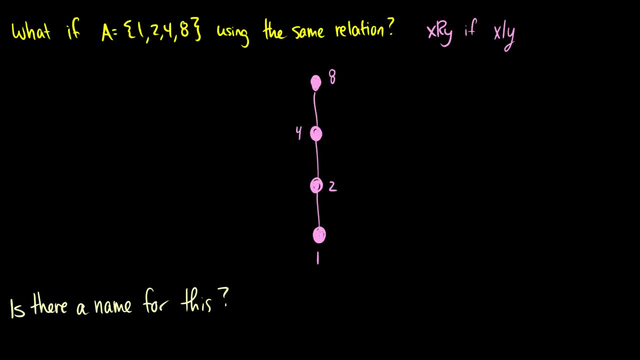 that is called a total order. Why is it a total order? Because we can arrange all of our elements in a straight line. If we can arrange all of our elements in a connected straight line, it's called a total order And that means that the elements are all. 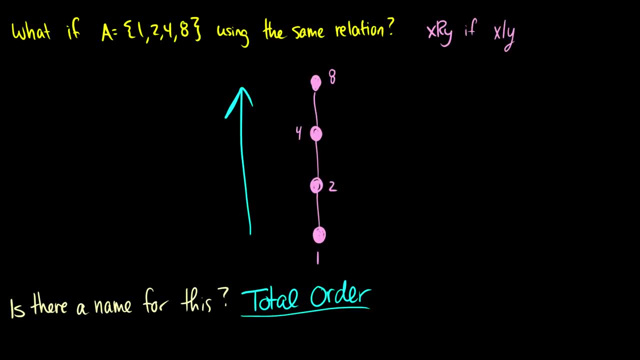 reflexive, anti-symmetric and transitive with each other. So this holds the same relations as it would before, but it's much more concise, much easier to look at And using this we can find minimum elements. we can find maximum elements. 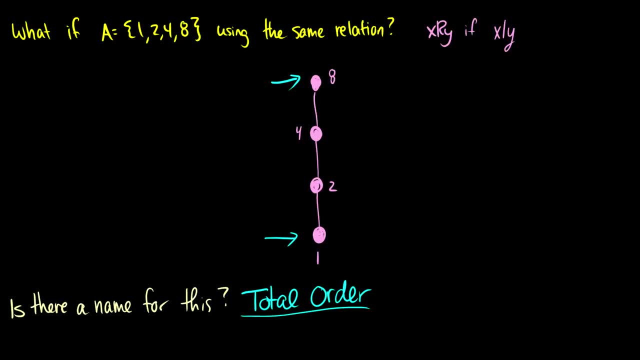 we can find some other least elements, greatest elements, but we won't get there, We won't cover that. Essentially, minimum element is the bottom, maximum is the top, least and greatest. So what can happen is you can have two bottoms in some graphs. 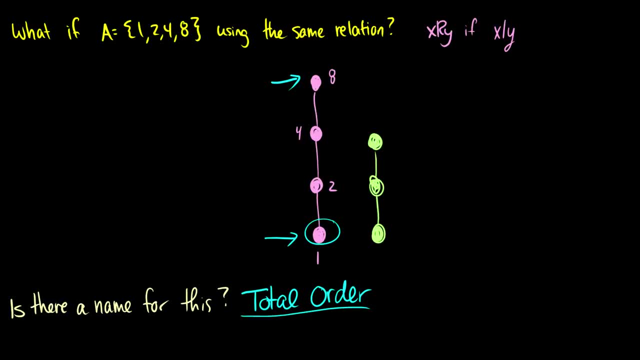 So we can have, say, two total orders as one partial order. It's not really called a total order, but then we'd have a difference between a least element and a minimum element. Or say in this, if we started with a zero and a one and two different things. 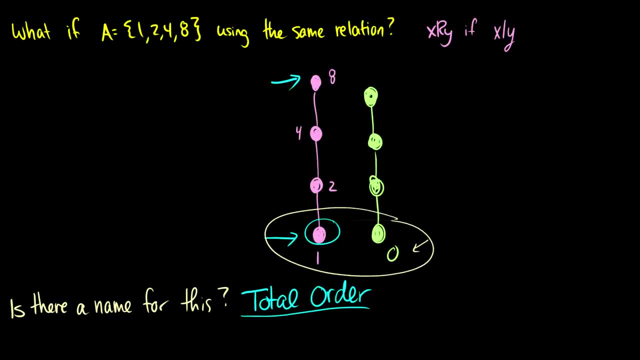 we'd have the minimum element being a zero, but the least element would be the pair one and zero, because they're at the very bottom. So that's some other terminology you might need to know, but it's generally not covered in a discrete math one course. I'm not sure. 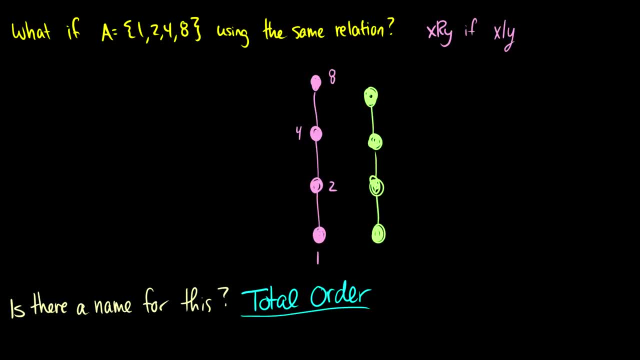 So at least it's not covered where the textbook I'm using is not covering it, So we'll just forgo that. Anyways, that is partial orders and equivalence relations. So hopefully you found that helpful. There's more material over at trevtutorcom. 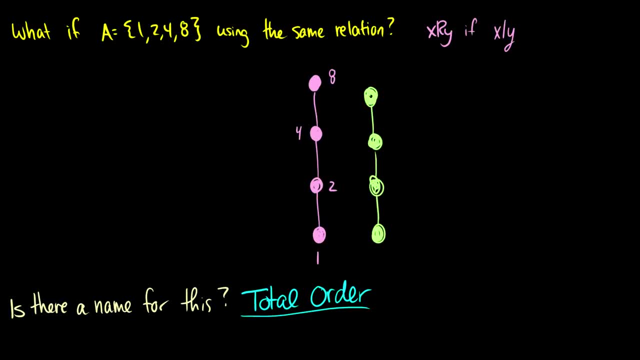 and I'm not entirely sure that on my midterm or final there are any questions on partial orders. But if you need practice, the book, I should probably write this at the end of every video for discrete math, but you can Google the book of proof.